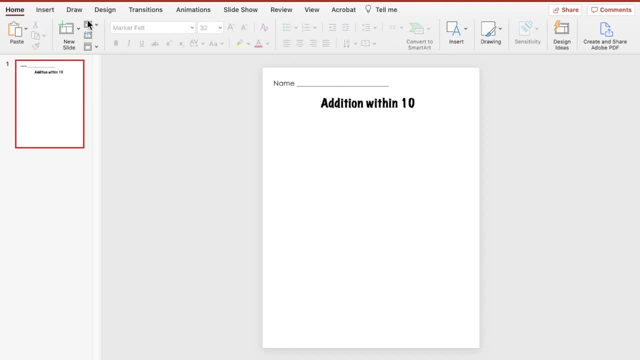 back and do our directions. So we're going to start on our first problem. So I'm going to insert another text box to do my number one: Change the font and the size And then make sure that it's in the right place. 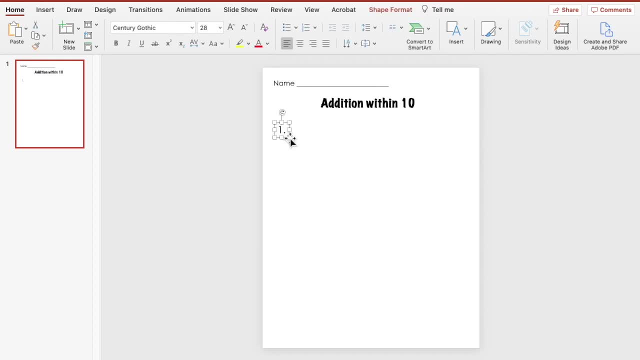 And then make sure it's resized. Okay, so there's my number, So I want to do this first page with pictures, So I'm going to go to insert. You can grab images offline or if you have some saved in your saved in a folder, I'm going to use the icons that come with PowerPoint. Click on icons. 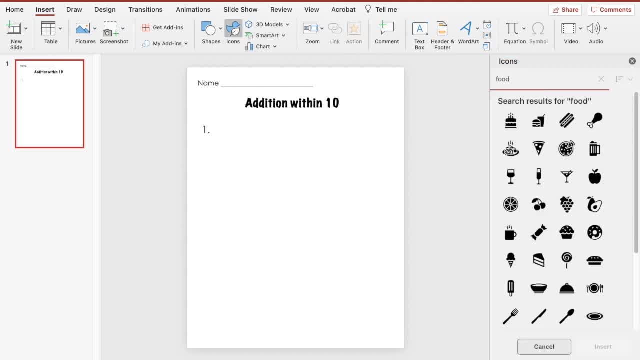 and then to get the apple. I'm just going to go to the food section and choose the apple and then insert. I'm going to move that into place, Then make it a little bit smaller, And then I'm going to double click it so I can change the color. 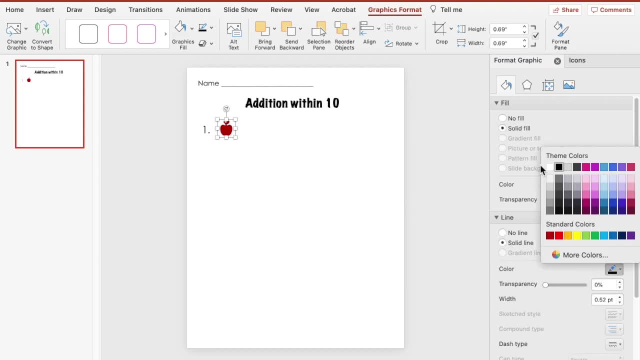 And then the line: I want to have it black. So the apple is ready. so then I want to duplicate it by hitting command d. You can also copy and paste, Get them aligned, And then I'm going to show that I want it to be a little bit bigger, I'm going to add a little bit. 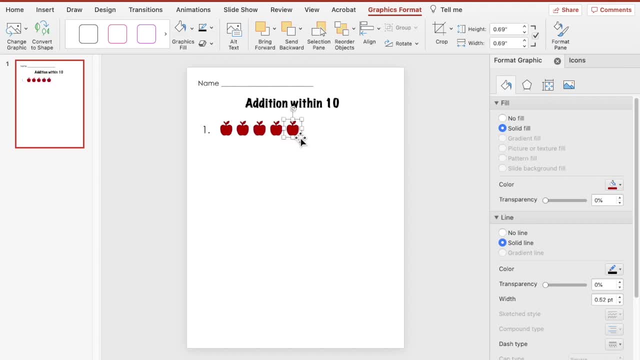 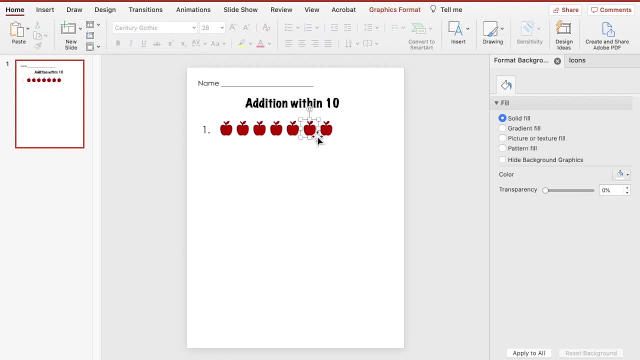 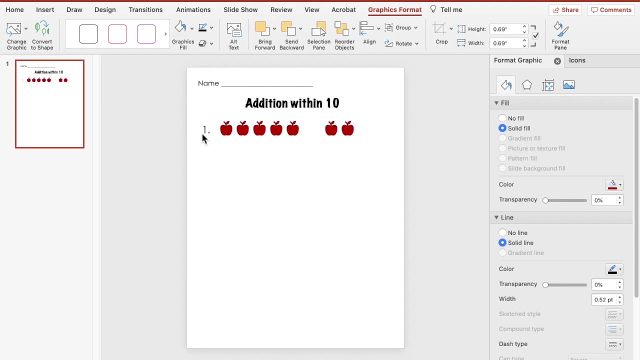 to duplicate. I want to do five on one side and then two on the other side, so I have one, two, three, four, five, six, seven. so then I'm just going to grab these last two and then pull them down. I want to pull this one a little bit closer to. 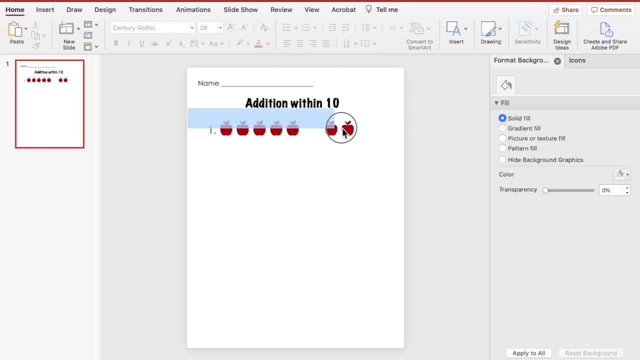 that first Apple and then select all of them and move them over just a little. so I need to add my plus sign and my equal sign. so I'm going to duplicate this text box around the one and then duplicate it again so I can do the equal sign those. 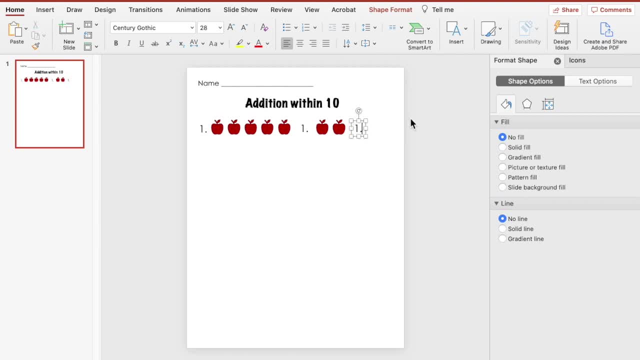 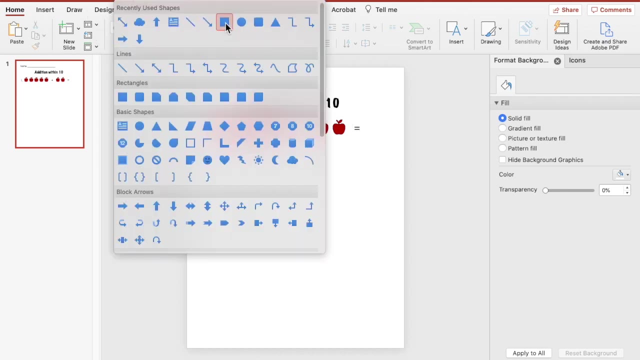 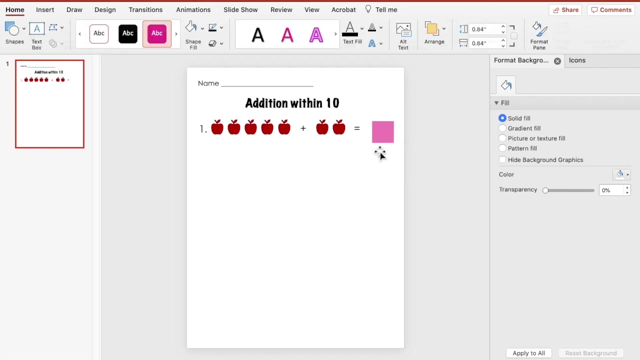 lined up and then change this one to the equal sign and change this one to the plus sign using my keyboard, and then I'm going to have the students put an answer in a little box. so I'm going to go to my shapes and draw a box. I want the width and the height to be the same and then it to be lined up. 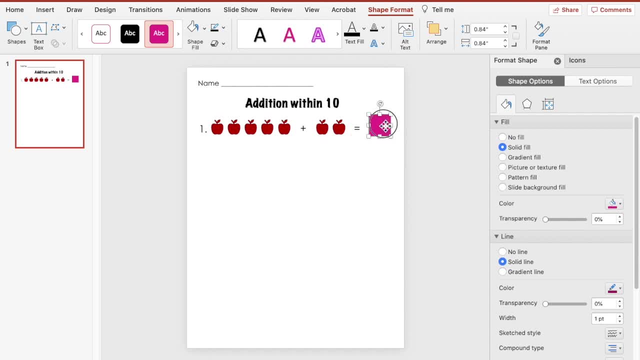 on the bottom, the same. alright. so for my box I need to get rid of the color. you can do no fill, do no fill. and then our line: we want to be black, and then I want to be thicker than that. so under line I'm going to go to width and then 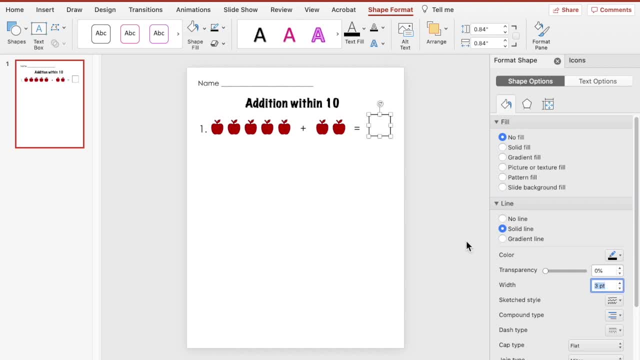 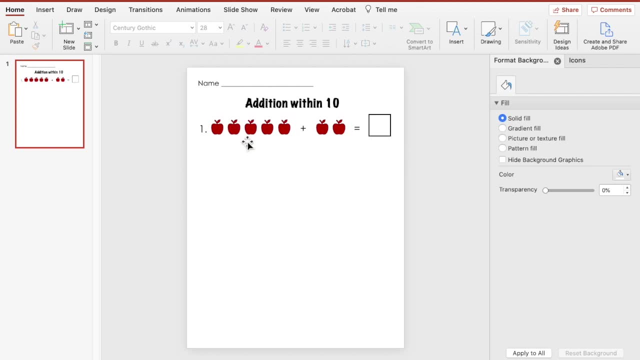 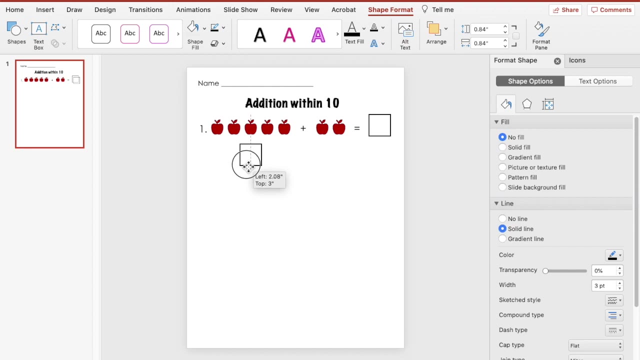 increase the thickness to one that I like. that looks good. so now I want to draw boxes under each section of the equation so students can write the amount that they count. so when they count the five apples, I want them to write the number five. I'm going to decrease the size of this box, or this. 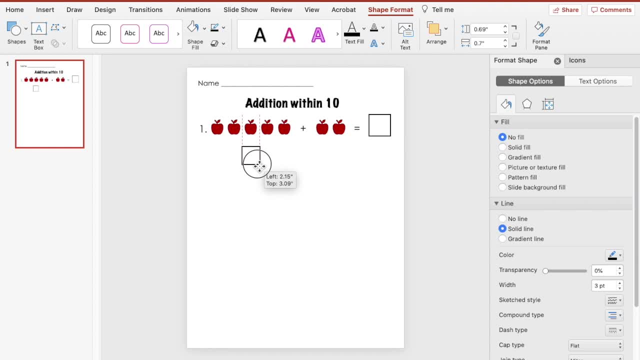 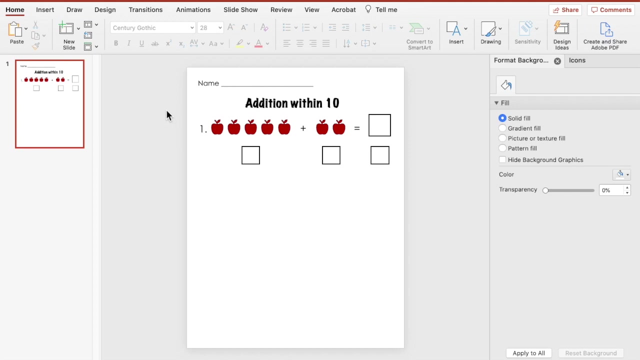 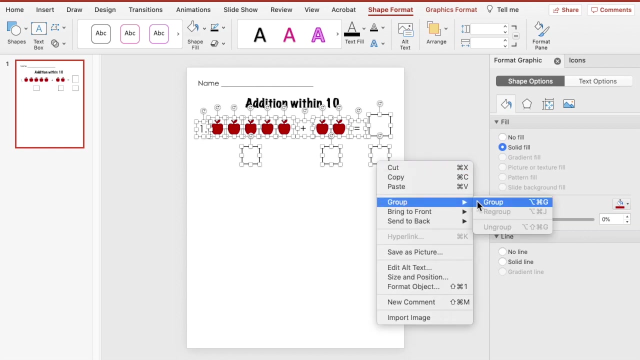 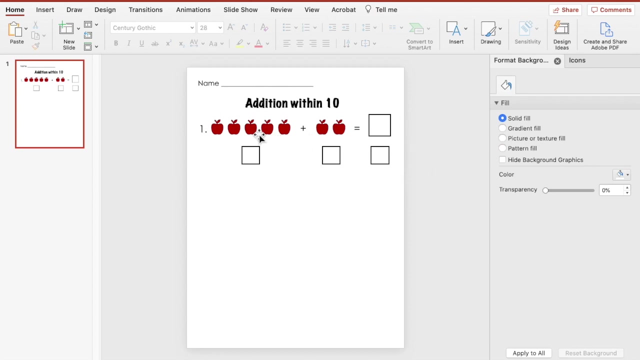 square and Center it and then duplicate it here and then duplicate this one and put it under there. I'm going to select all of these two together and then group them. remember, you can right click, group and then group together and then I want to outline to go around the entire problem. so I'm going to come back up to the 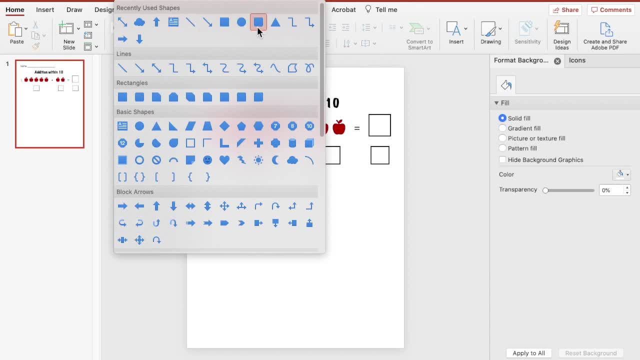 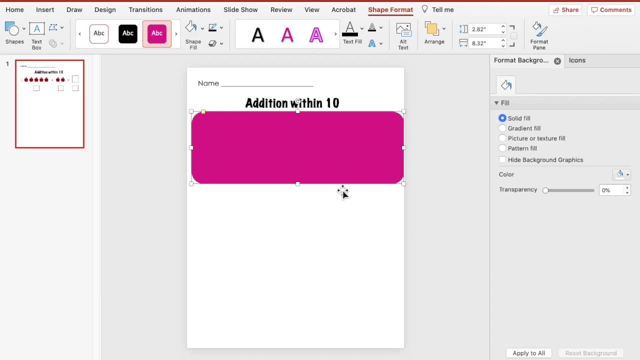 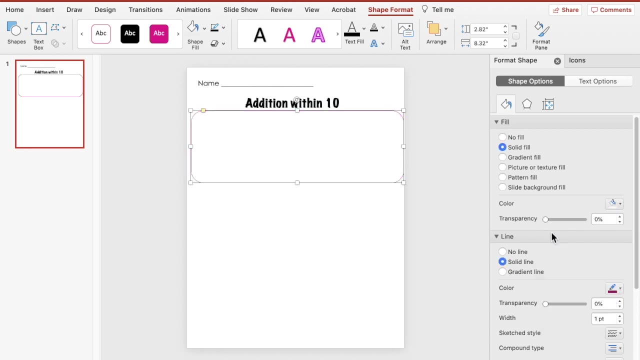 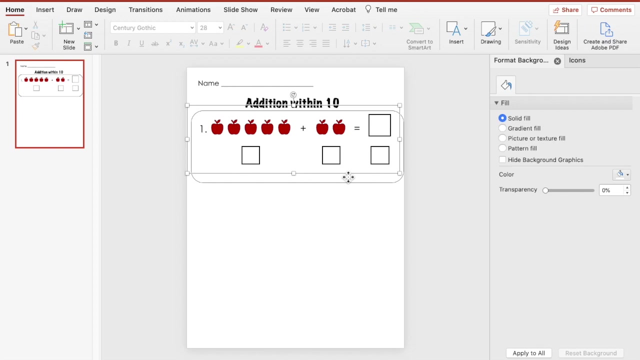 shapes and choose this square with like rounded edges and go around the whole problem. you can move it up a little bit. I'm going to change the fill color to white and then the outline to black, and then I'm going to right click on it and send to back so I can see the problem. I'm going to click the actual problem. 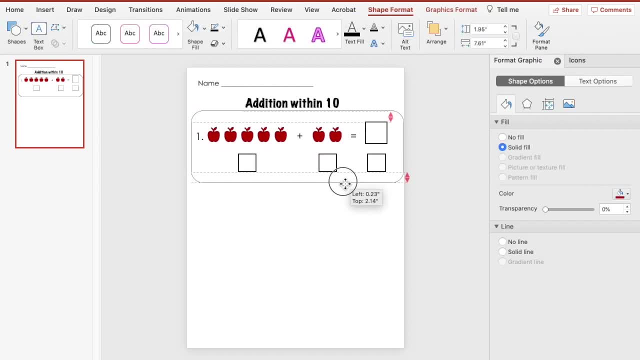 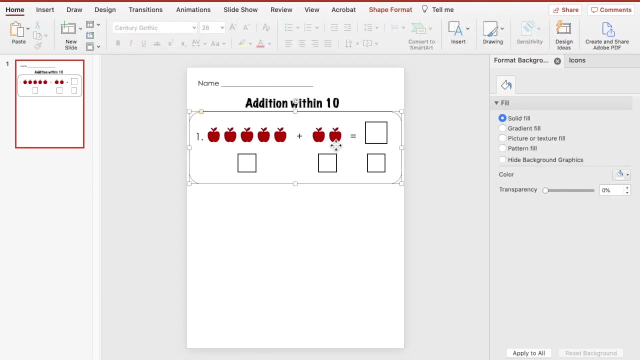 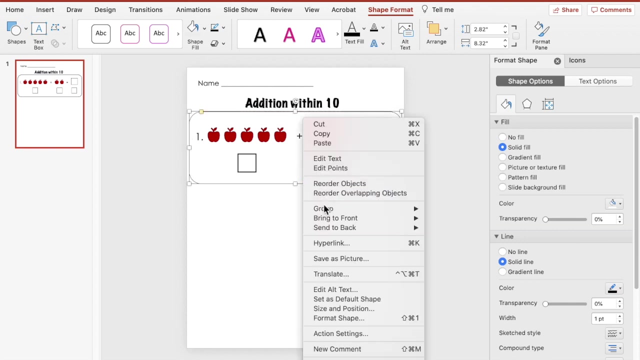 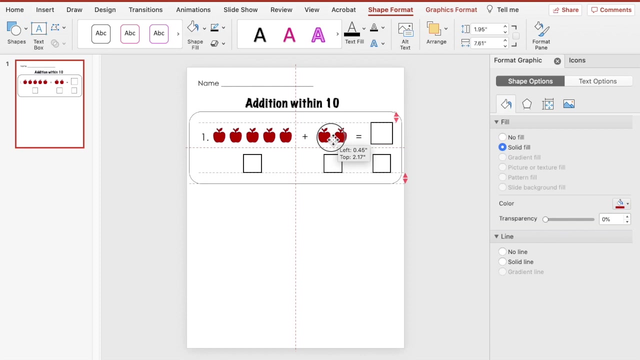 and move it down and try to Center it within that square or that shape, that rectangle. let me Center the rectangle and then I can Center the problem. okay, let me send this back again, send backwards, okay, so I want to move that and Center it. okay, so that looks great. now what I want to do here is make this: 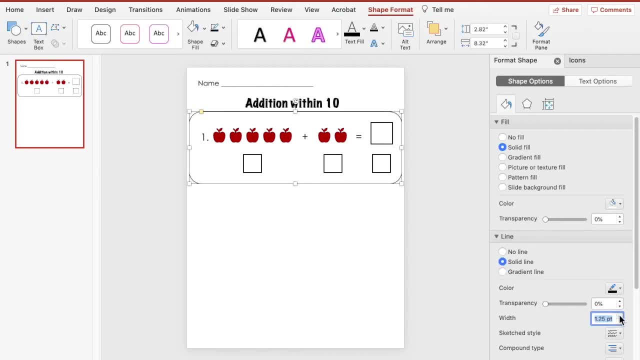 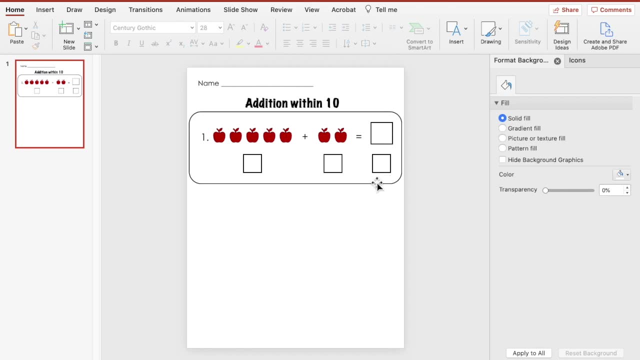 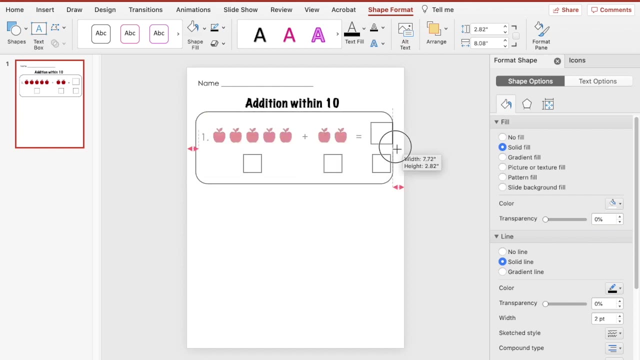 outline just a little thicker, so I'm going to come back to the width for that and I like it at two. I like it at two. so let's bring it in a little. and I want to bring it in because I want to put an outline around the entire page, so I 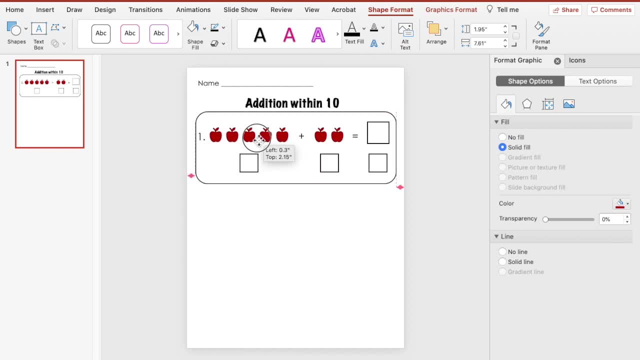 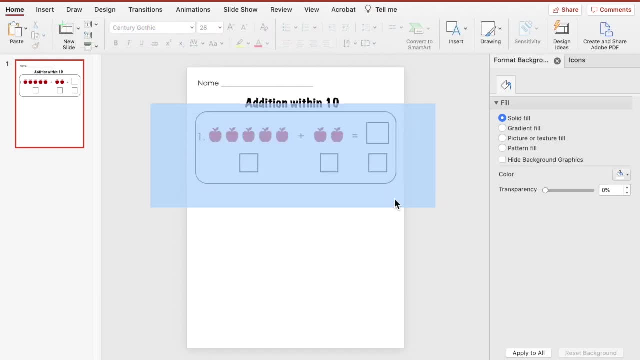 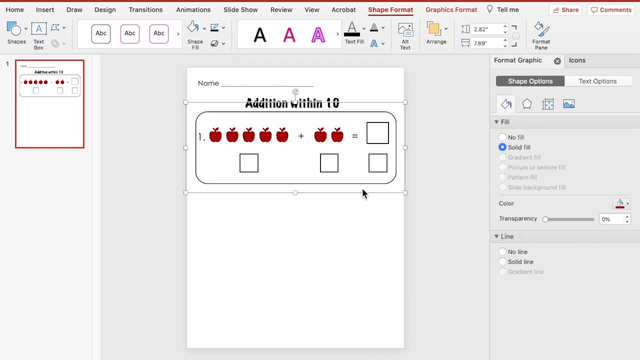 don't want this to run into that outline. let's move these over. I'm going to select all of it so that I can group all of it. so I have the problem and that rectangle group together. it's not a rectangle because the sides are curved, but that rectangular shape I'm 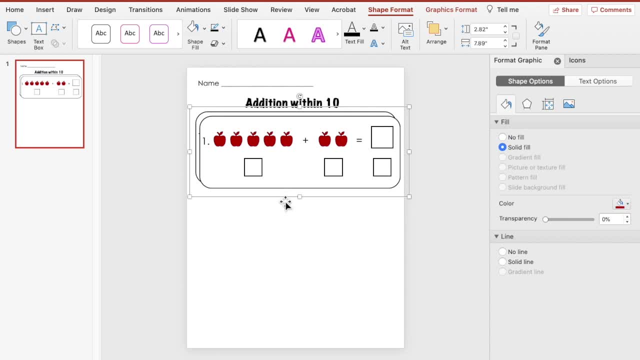 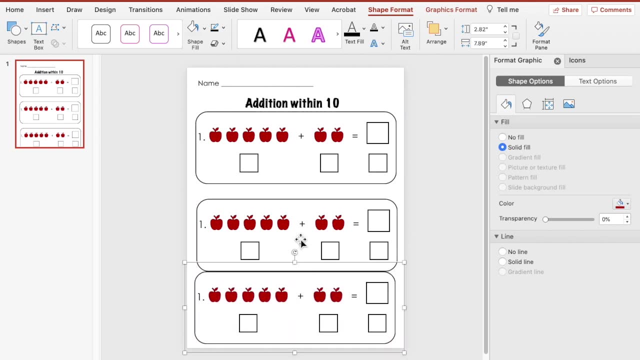 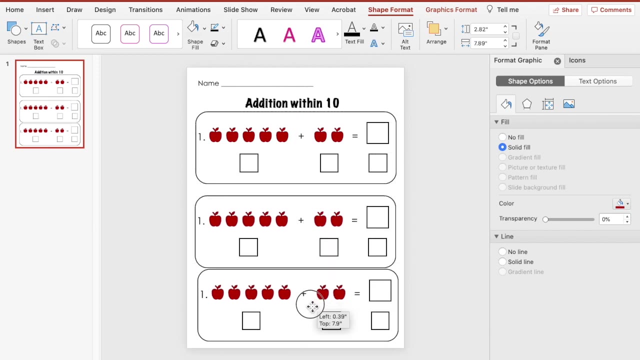 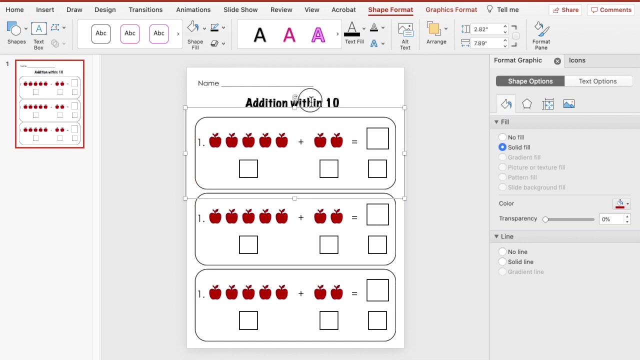 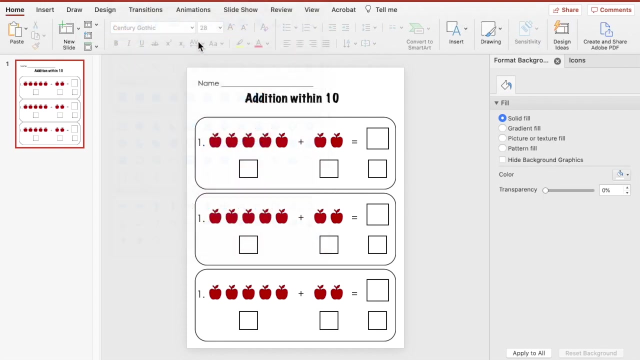 going to duplicate it and bring it down here and then duplicate it again and then just move them so they're distributed kind of evenly, like this. I'm going to equally See there's a center that's not centered and I want to leave space for the directions that I'm going to add. So let's go ahead and add in a rectangle to: 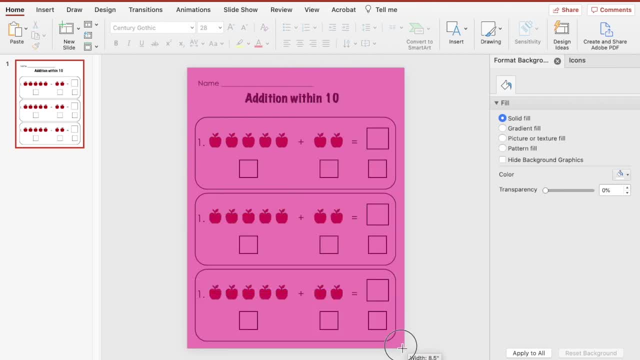 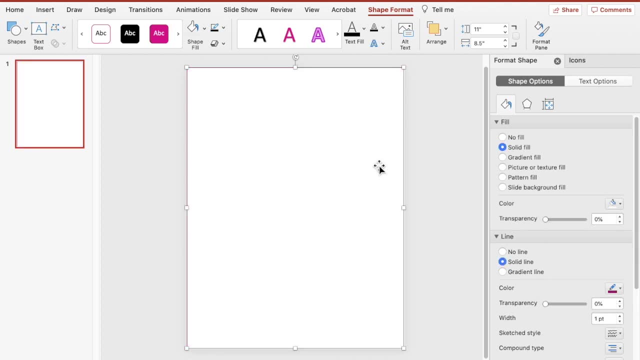 create the outline. So I start by adding a rectangle and then I make the fill white and I send it to the back- Well, not backwards, but send it all the way to the back- And then for the line, I want to make the line black and then increase. 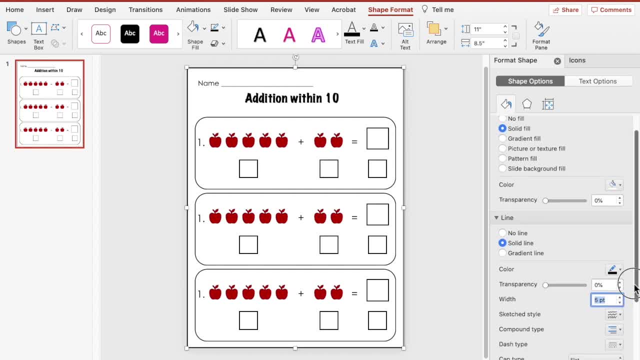 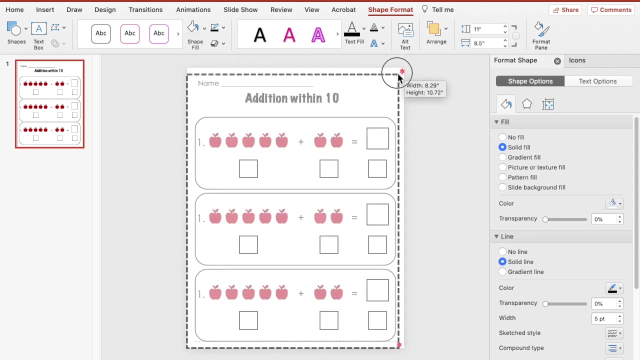 that width to about five And I'm going to change the dash, the solid line, to like a dash, Or let's do the other dash. I'm going to bring it in a little bit. I'm going to hold the shift key down so the dimensions kind of stay similar to each other. And then recenter, 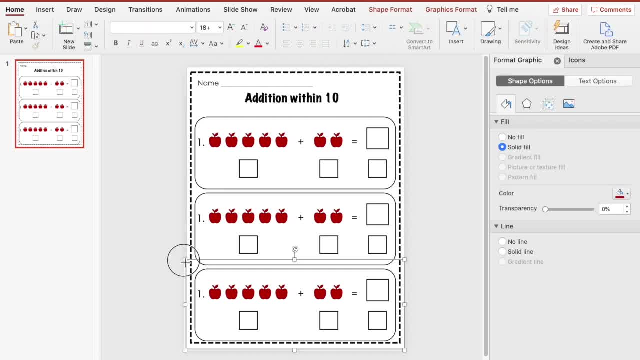 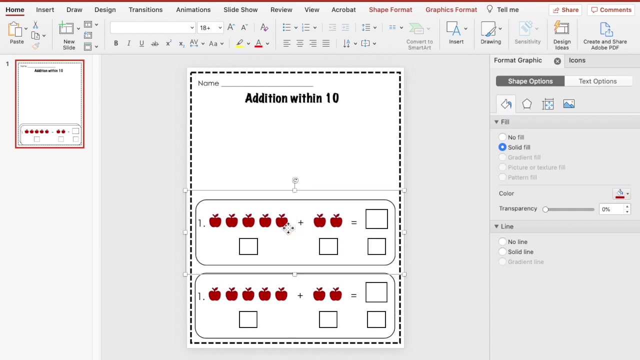 that outline. Let's shrink our problems just a little So they're not running into everything. I can delete these and then duplicate this one, since it's still the same, And then duplicate that one, And then I have room for my directions. 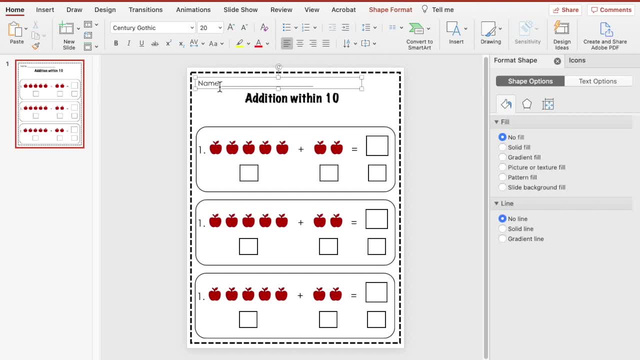 So. So let's take the name and duplicate our name and bring it here. I'm just going to erase what's inside. I'm going to add: make the directions bold directions, All right, so the last thing we need to do is change the second and third problem. 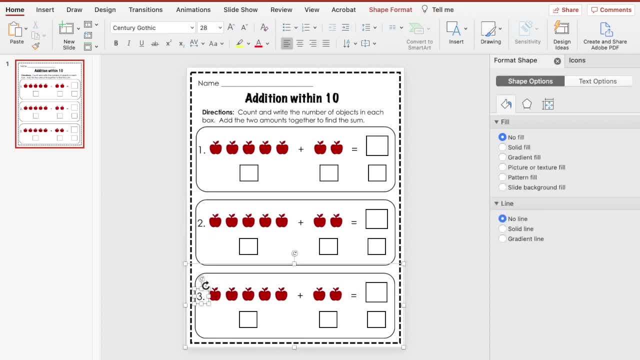 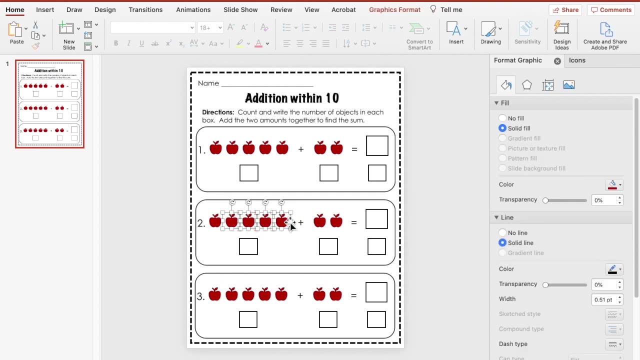 So we're going to change that to number two and then change this to number three. So I'm going to ungroup this one, this set, ungroup it twice, And then get rid of these other apples. And I'm going to click on this first apple, right click it and then go to change graphic and then from icons. 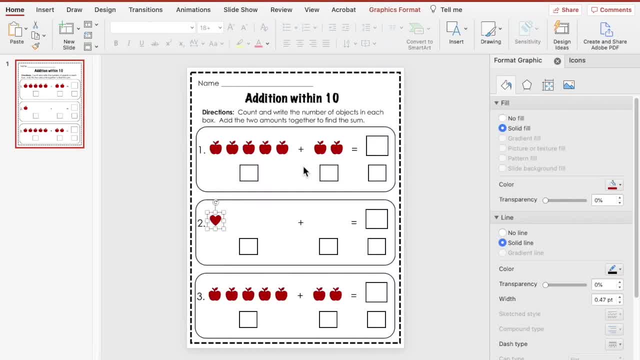 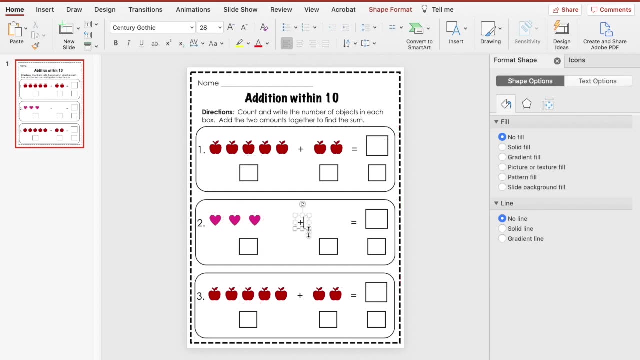 So I found a heart that I want, so I'm going to insert that, change the color and then this time I want three plus three. so I'm going to duplicate that and resize it and then bring the plus sign over and then duplicate that set and that works. 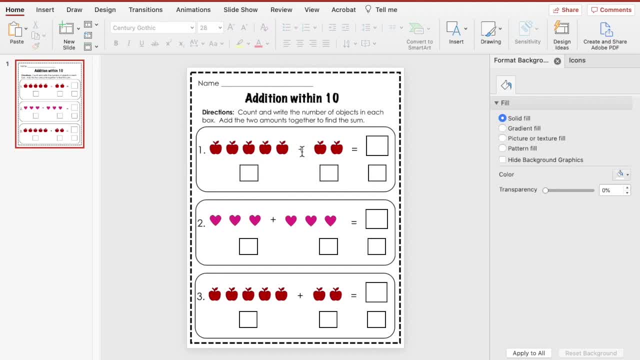 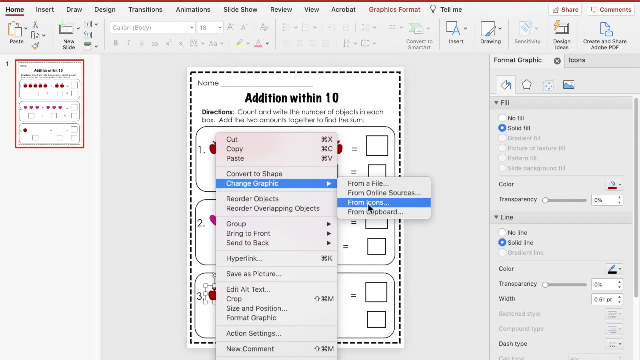 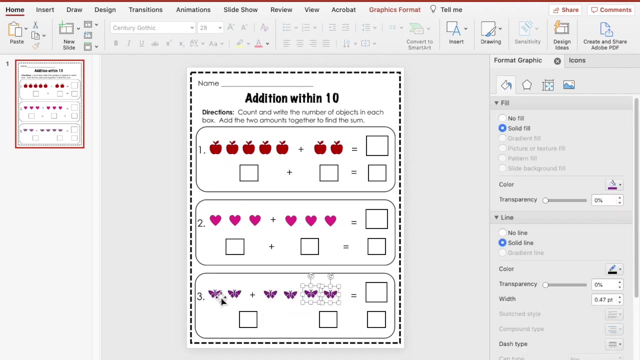 So I just realized I didn't put the plus sign Here in the equal sign here. so we're just going to duplicate that. So this sheet is done. so let's duplicate our sheet. So we're going to kind of use the same heading. 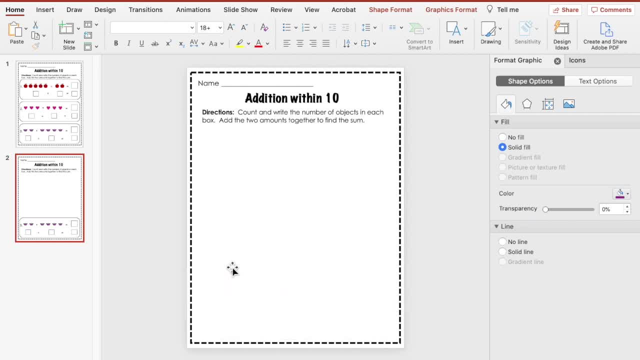 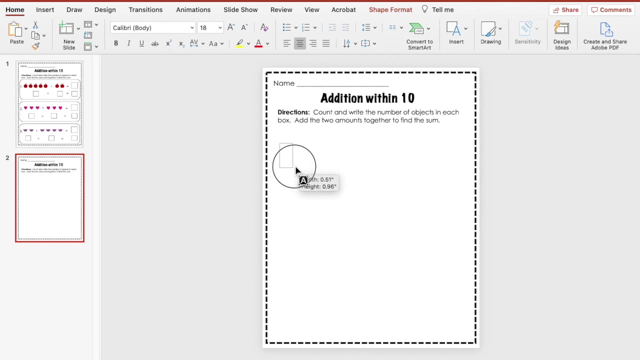 We're going to get rid of our boxes, our three boxes, because we're going to do just equations without pictures. So I am going to insert a text box for the number one- Let's change our font, Number one- And then we are going to duplicate that text box to draw, to write or create our equation. 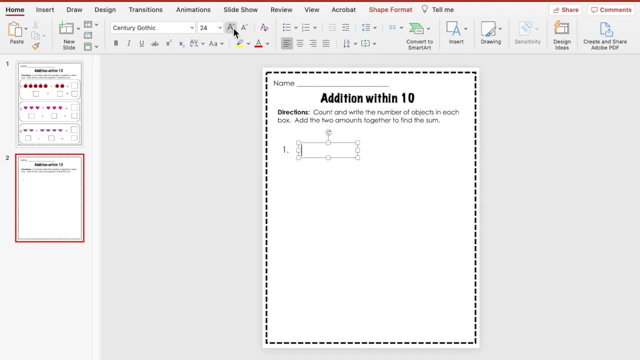 So let's delete the one. I want to increase the size one. Let's do six plus seven equals. stretch it out so we can get a bigger size, Make it a little larger and then get it closer to that one, but not too close, where it's confusing. 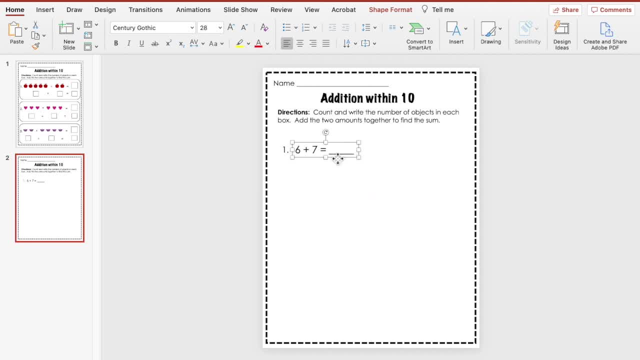 And then bring in our text box. So then we're going to duplicate. Well, I'm going to take that and hit the, grab the one and then group those together and then hit duplicate and move this second one over and change the number out to number two and change the problem to four plus nothing. 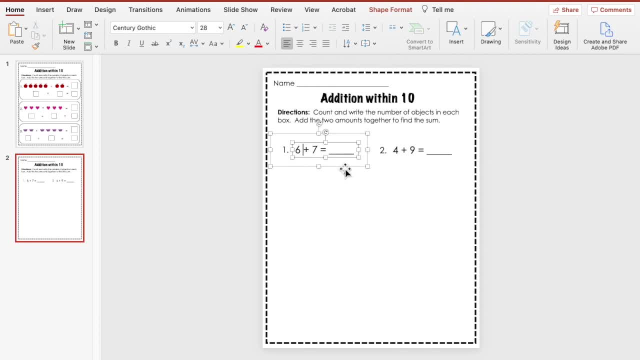 So I'm going to then duplicate both of these And There's the other two, and then I'm going to reveal the other two. So you have my three boxes together. They're selected. So just to remind you of duplicating, you can copy and paste or you can on your keyboard. 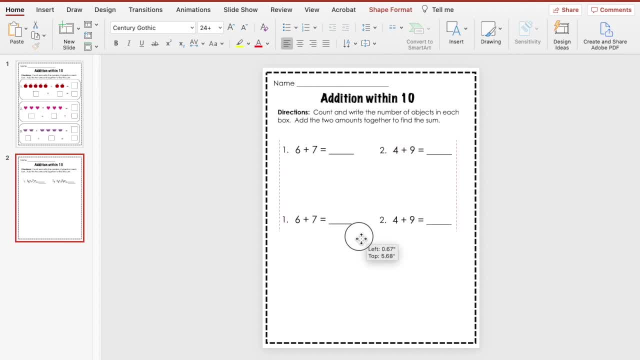 You have a Mac, hit command d, or if you have a PC, hit control d to duplicate. And I'm going to leave some space between the problems because I want the students to show their work. So then change out our last problems to 5 and 6, and then let's make this one 2 plus. 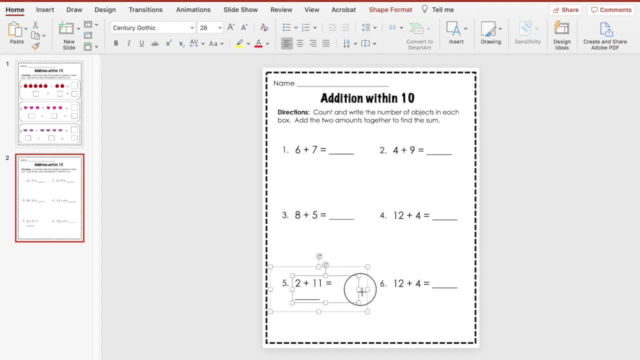 11, and then this one, 16 plus 3.. So, as you can see, we're not within 10 anymore, we're now within 20. so I'm going to change the title to addition within 20. and then for the directions, let's actually bring our equations. 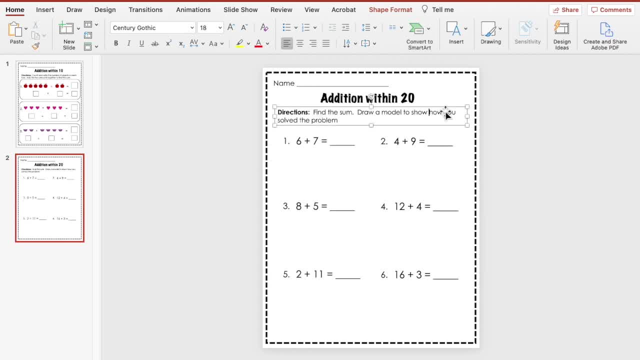 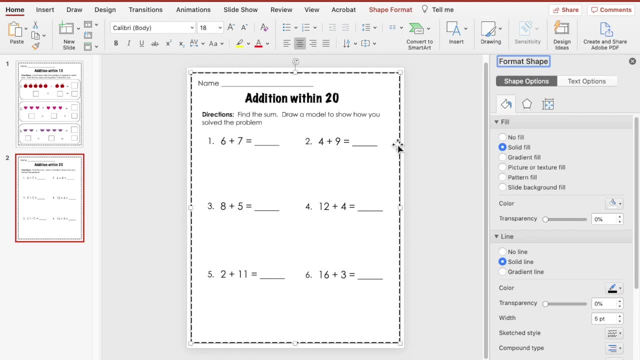 up just a little and our directions can come down a little. So for this one, let's change our line, our outline. So instead of a dotted or a dash we're going to have a semicolon Solid line, but then let's change it to like a little crinkly line. I think that's cute. 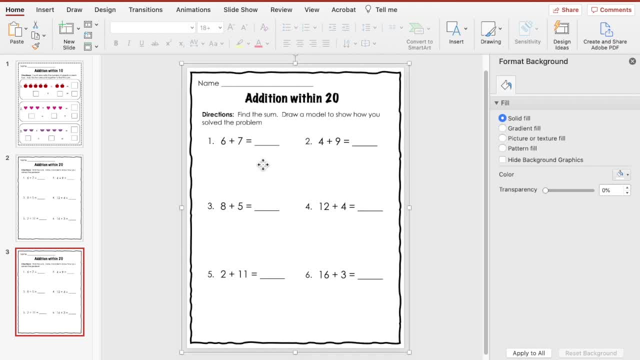 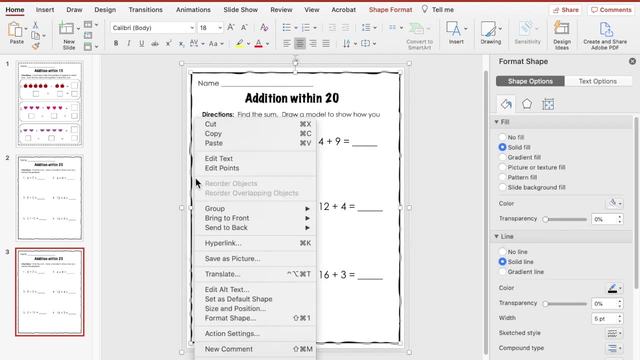 We're going to duplicate that second page to make our last page and we are going to do a few vertical problems. So I'm going to get rid of all of the problems. let's ungroup. it's very easy. It's very easy to ungroup. 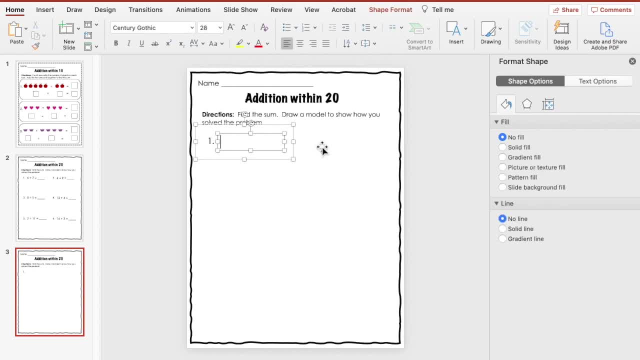 So let's do- I'm going to tab over. let's do 350, enter the plus sign and then 48. So then I'm going to go in front of the plus sign and hit tab. that's too far, So I'm going to backspace and then just use the space bar to go over where I want it to. 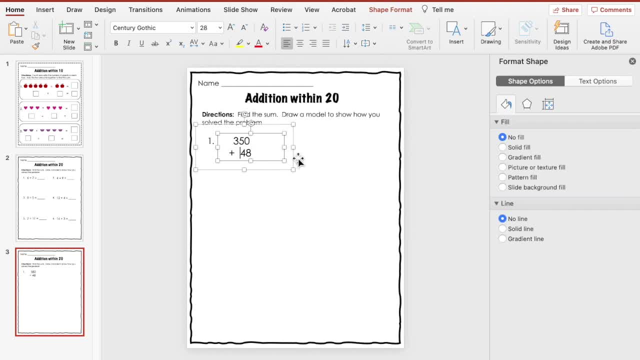 where I want it to be and then in front of the four, I'll go over one. okay, so that they're pretty lined up. now you can select that bottom section and go to the underline button and have it underlined that way, or let's undo that you can go. 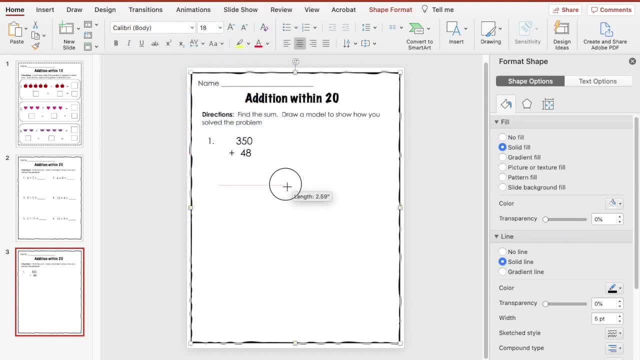 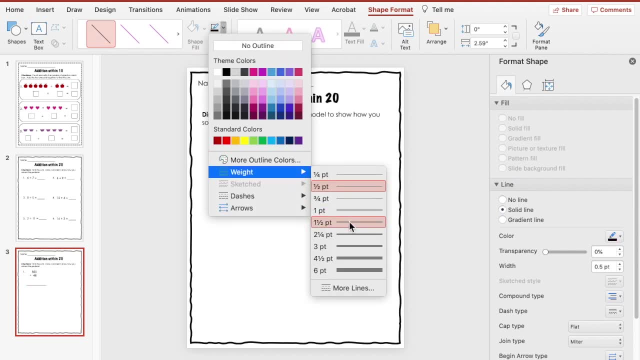 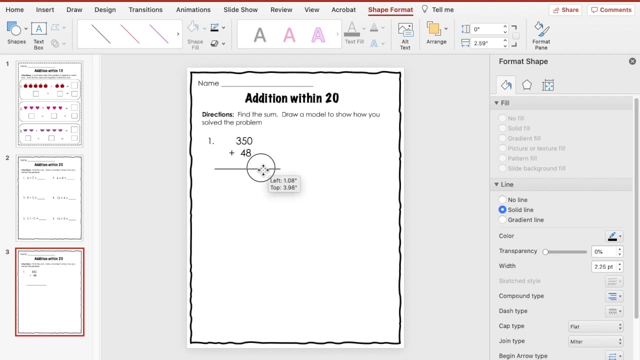 to your shapes and draw a line, however long you want it to be and however thick you want it to be, in whatever color you want it to be. so let's increase the weight. it's a little bit more. that looks good. that's way too long. let's bring it. 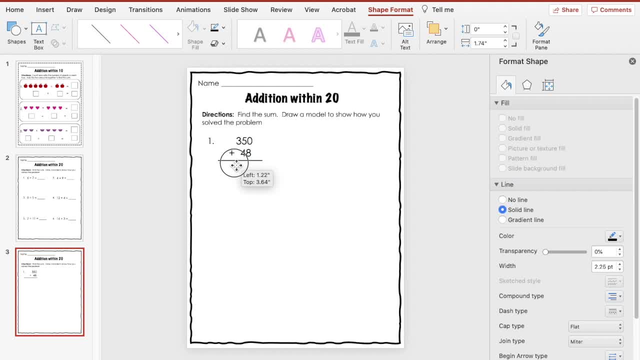 in some, bring it in a little bit more. okay, so that works. let's bring in our number, number three, and then we're going to go ahead and make sure that we're going to make sure that we're going to make sure that we're going to. 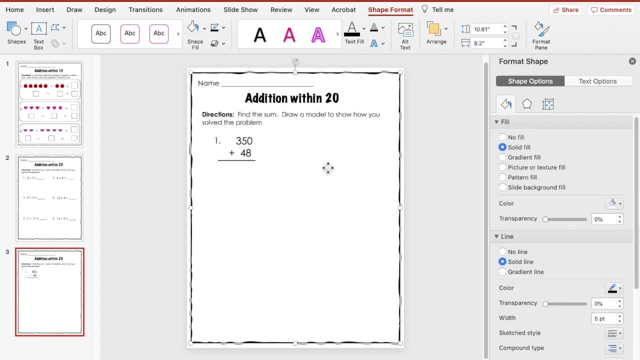 number one, just a little bit, and we are going to make sure that line is selected with our problem and group them together and group: select the equation and hit duplicate and bring that over here. and select the equation and bring that over here. and 0 for number two. lets change it to 934 plus 200 and then we're going to. 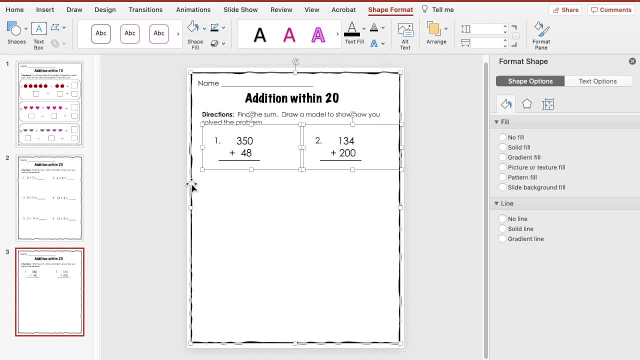 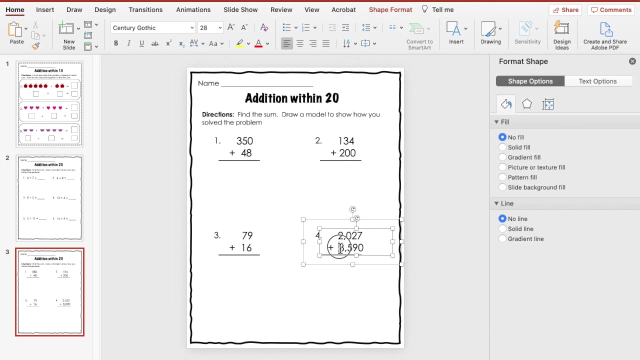 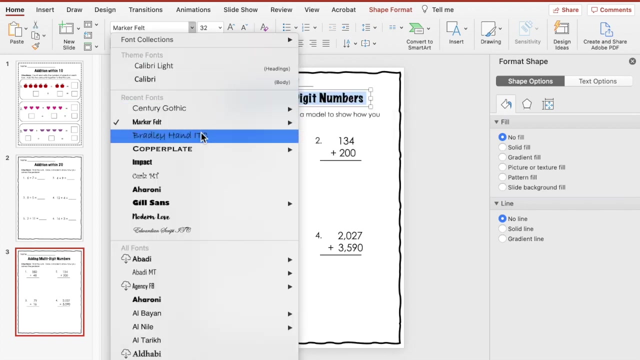 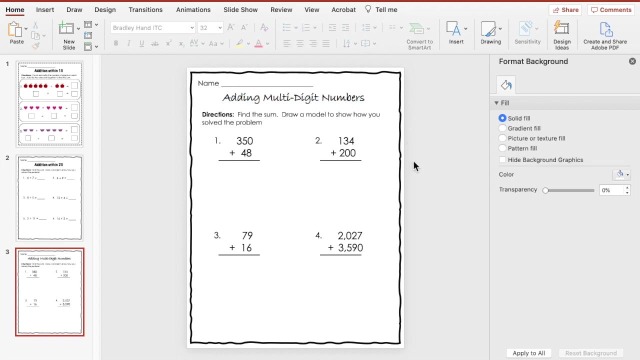 0 for number two. lets change it to 934 plus 200, and then we're going to duplicate both of them and I just want to do a total of four. duplicate both of them and I just want to do a total of four. Let's change our title so now we're not within 20,. let's make it bold and let's change our. 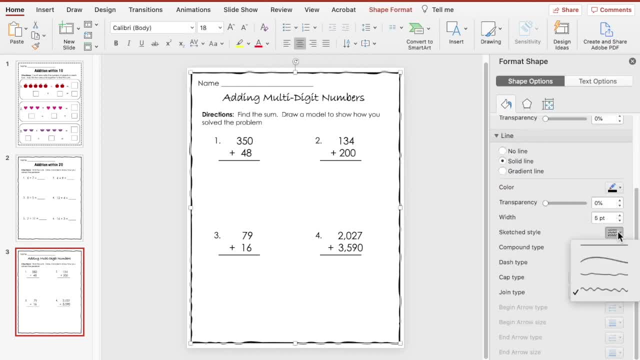 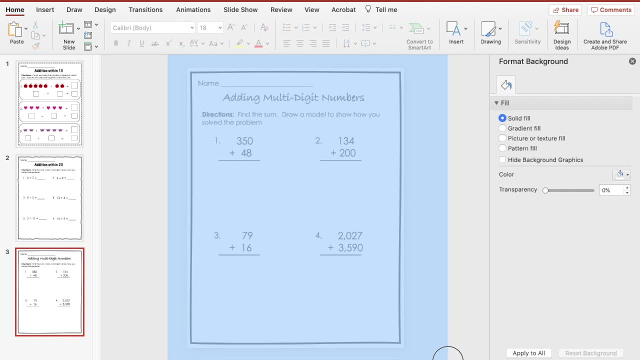 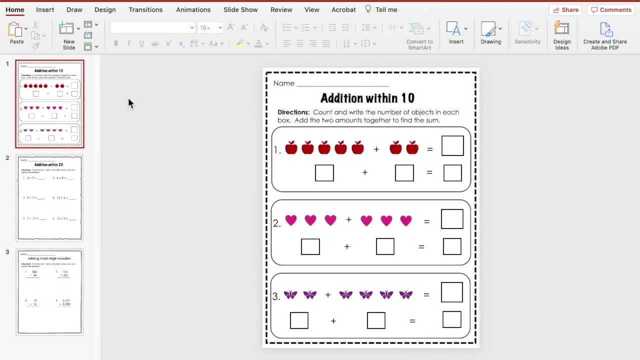 border. let's go curved- that's a little different than the last one- and let's select the entire page, right click and group. so what I want to do now is insert my name at the bottom, or my website name, so if someone wanted to find these worksheets, they can come there. 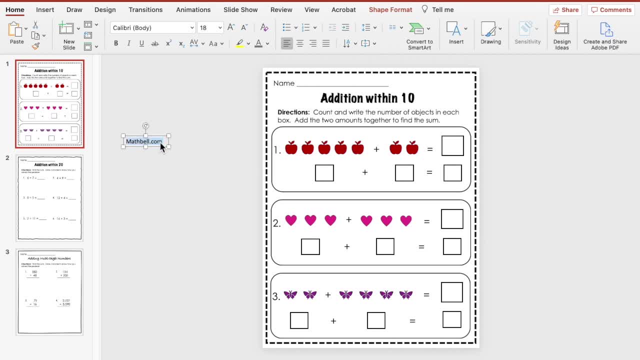 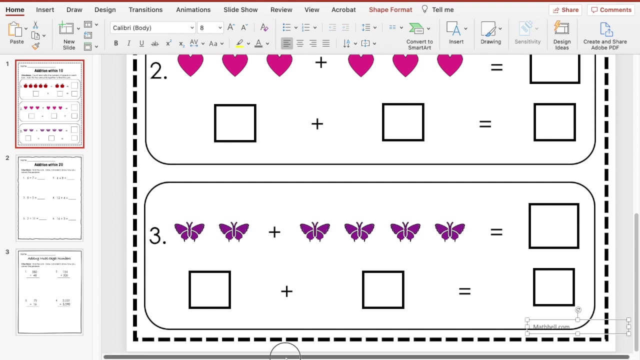 let's make it bold, Let's make it smaller, and when you're creating yours and if you're sharing it with other teachers or families, definitely put your name at the bottom, if you choose so. so let's change the color to a gray and then make it a lot smaller so it fits. let's zoom in then.